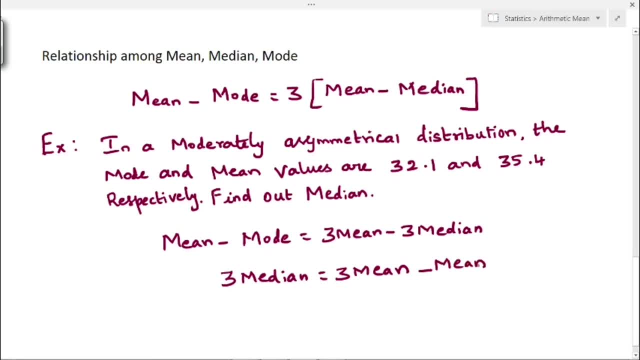 So if you take it to the other side, it will become minus mean. And I am taking this minus mode to the other side, So it will become plus mode. So this formula will become 3 median equal to: I am going to subtract these two: 3 mean, minus mean. 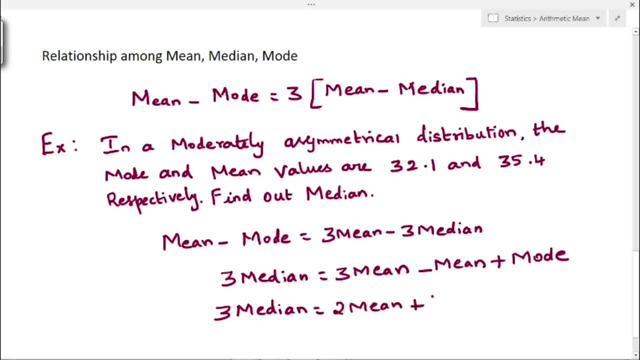 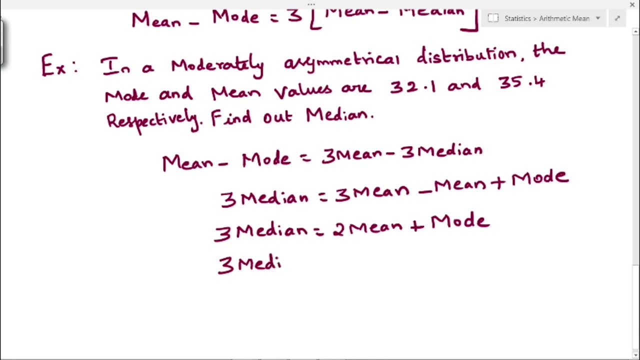 That is, 2 mean plus mode, Because we want to find out the Value of median. So I am taking mean value to the left hand side and remaining values to the right hand side. 3 median equal to 2 into mean value. 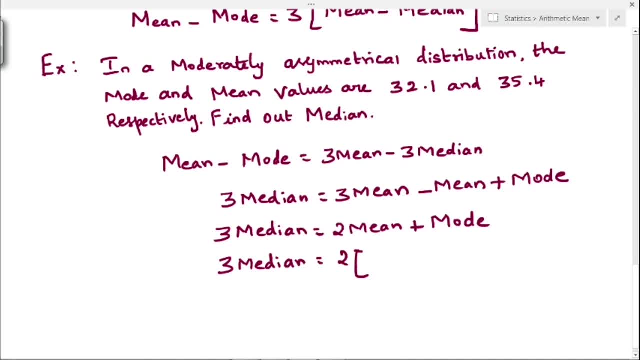 So in the given problem mode and mean values are 32.1 and 35.4.. So mode value is 32.1 and mean value is 35.4.. So I am going to substitute this, So mean value is 35.4.. 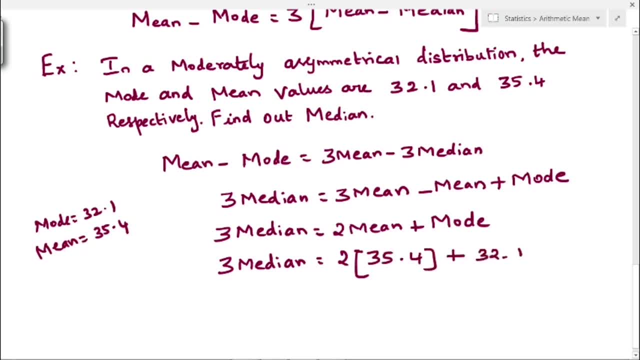 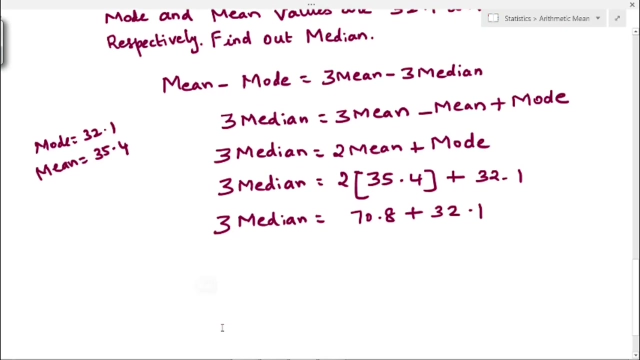 Plus mode value is 32.1.. So 3 median equal to multiply this 2 inside 2 into 35.4.. So answer is 70.8 plus 32.1.. So this is nothing but 3 median equal to 102.9.. 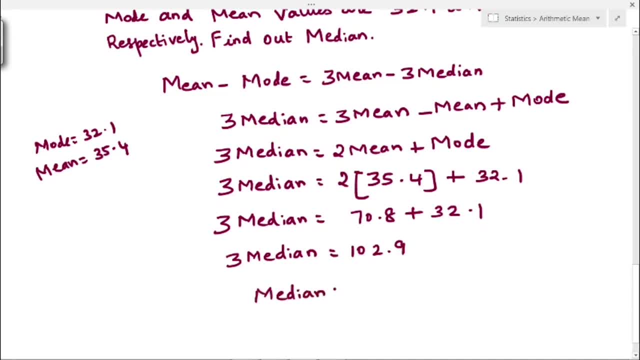 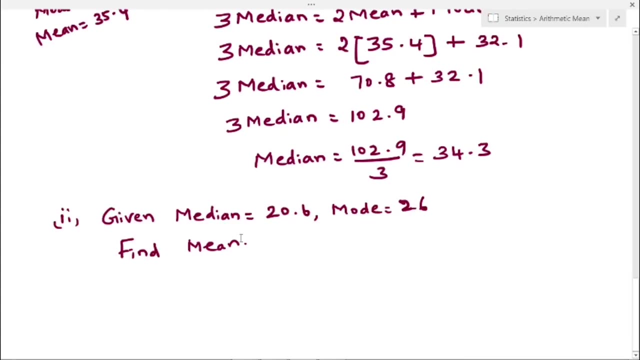 So we want to find the value of median. So median equal to 102.9 divided by 3.. So that is nothing but 34.3.. So this is the value of median. We will see an another example. 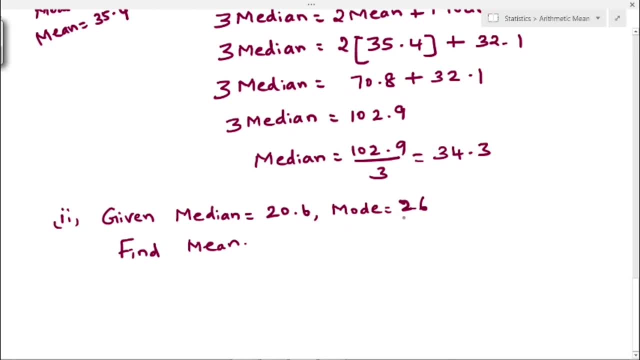 So in this example, given median is 20.6, mode is 26 and we have to find mean. So again, we have to use the same formula, So we have to use the same relationship, that is, mean minus mode equal to 3, mean minus 3 median. 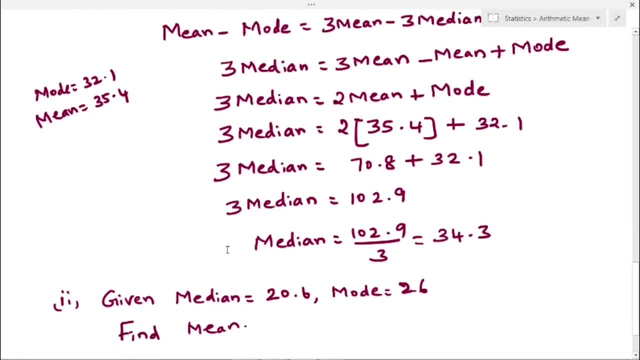 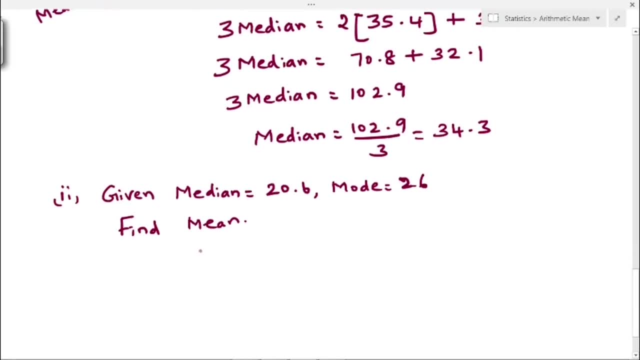 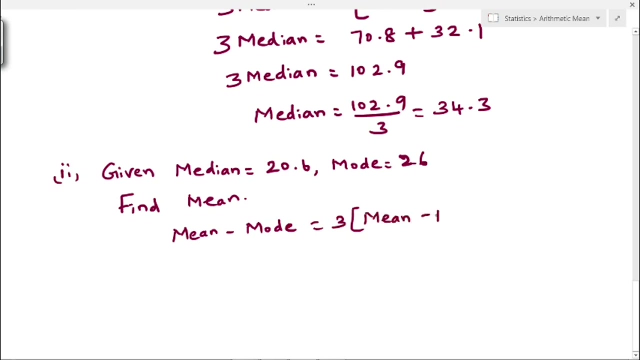 We want to find the value of mean, So we have to keep the mean value in the left hand side and we have to take the remaining values in the right hand side. So the formula will become mean minus mode equal to 3 into mean minus median.